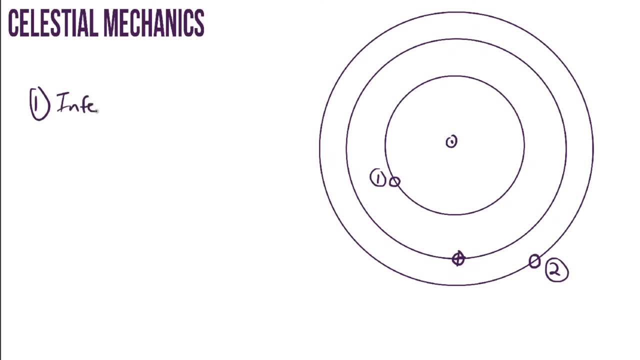 closer to the Sun than the Earth. these planets are called inferior planets, And then any planet that orbits further away, like planet 2, is a superior planet. Okay, notice, from the Earth's point of view, an angle is made between the Sun and the planet. Here we go, This angle, we're going. 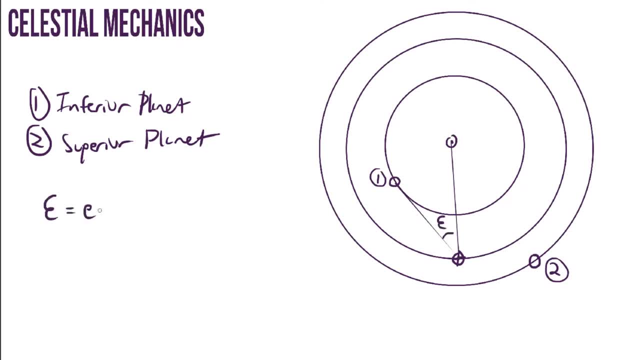 to represent with epsilon, and this epsilon is called the elongation between two planets. There are some elongation values that have their own names. When the elongation is 180 degrees, we call this opposites. When it is 90 degrees, we call this quadrature, And when this angle is 0 degrees, we call this: 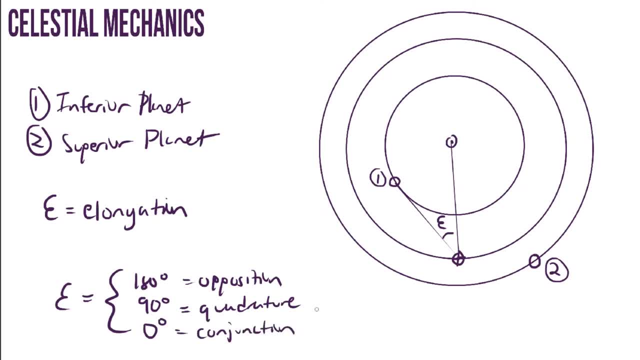 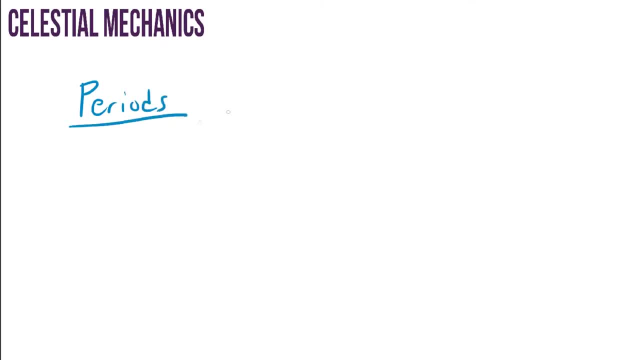 conjunction. The next thing I'm going to talk about are periods, which is essentially the amount of time it takes for a system to return to a certain state. The two that we care about are called sidereal and synodic periods. So a sidereal period is the time it takes for a full rotation of the Sun. 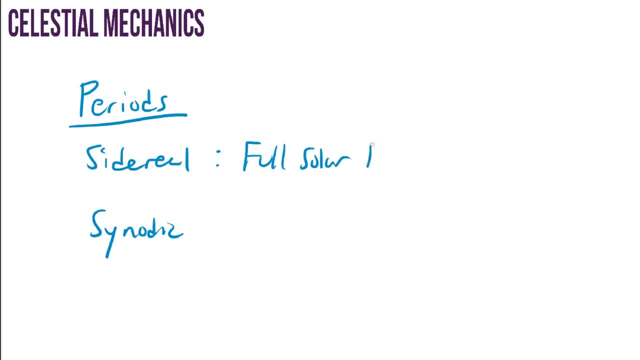 And a synodic period is the time it takes for a planet to reach the same position relative to the Earth. So, for example, a synodic period would be the time it takes for a planet to go from one opposition to the next relative to Earth. 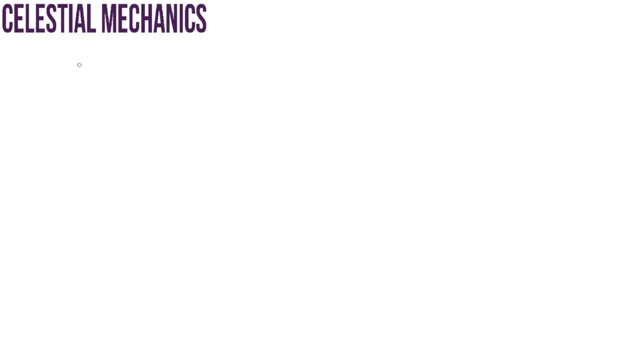 So we know that Earth orbits around the Sun. it completes a full revolution in one year. So we can say that it travels two pi radians in E, where E is equal to 365.25 days. Any other planet is moving with an angular speed of two pi radians over P. 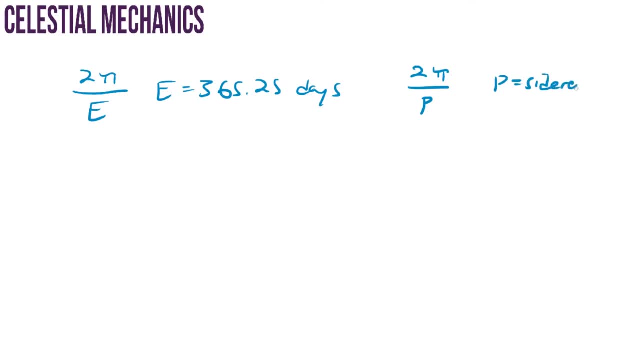 where P is equal to the sidereal period of the planet. Let's now say that S is equal to the synodic period for a superior planet. We can now say that the superior planet traveling from B to C along this route makes some angle X.